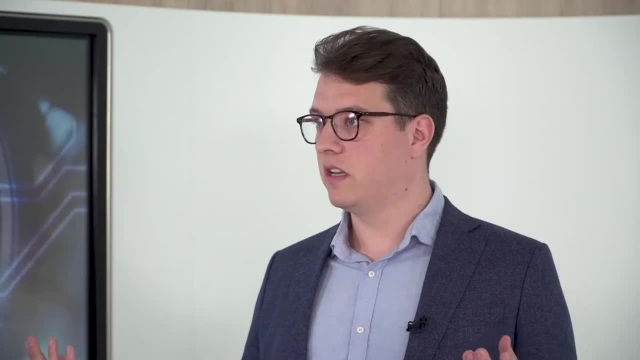 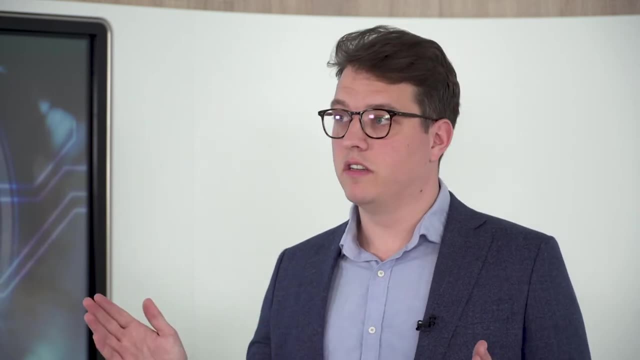 2021, they're talking 7.1 billion devices connected within buildings. The scale is just getting huge and we're not used to scale in this industry. It's very small amounts of data in terms of data analytics. So this is how some really smart people in the 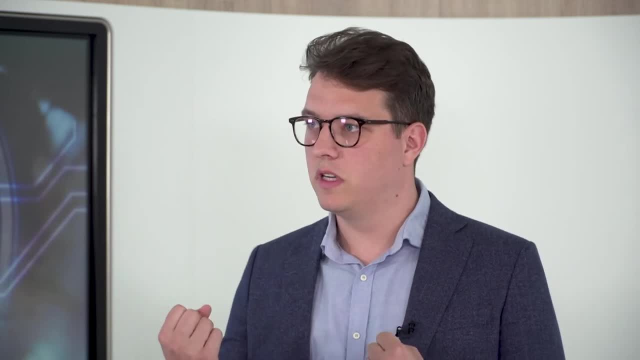 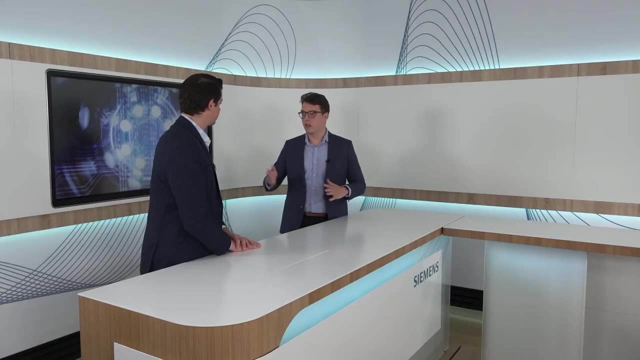 industry came together and said: how can we solve this? How, as an industry, can we solve it? Because it's not through a naming convention, because that loses all value once you leave one building to another, let alone another country, Another company, another system. 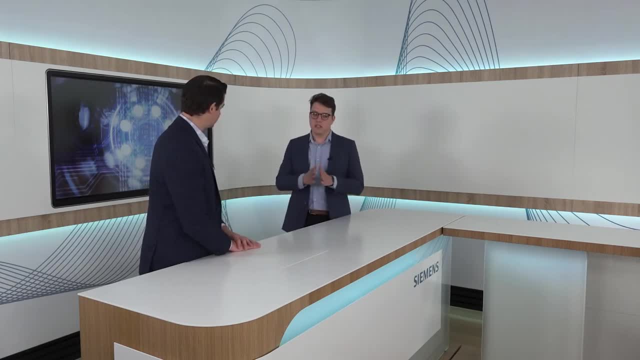 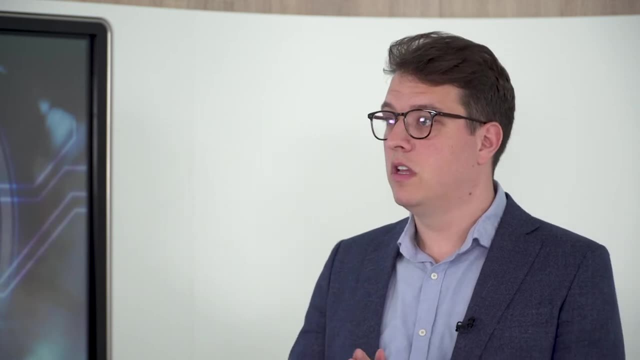 Another person installing the equipment, It does change dramatically. This allows us to say how can we universally solve this problem? There's a great committee coming together now for ASHRAE and some of the people from BACnet and another tagging system called Haystack and 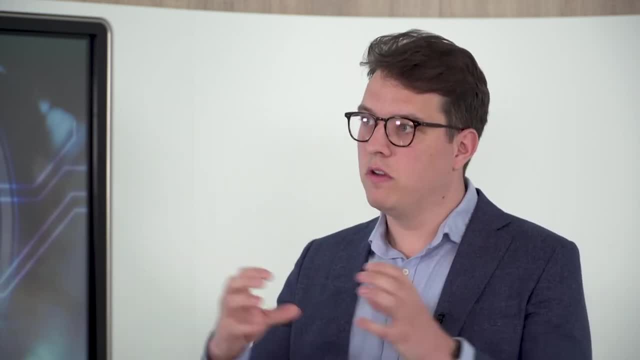 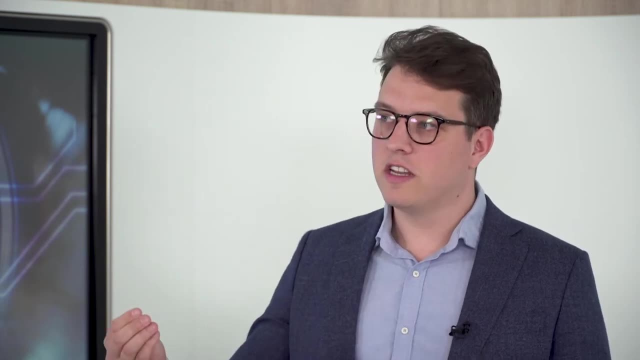 Brick Schema. They're coming together to say how can we create a unified approach, How can we put something to our industry that can help them solve problems? And it's such a great initiative because it's done from a. we need this so we can make better products. 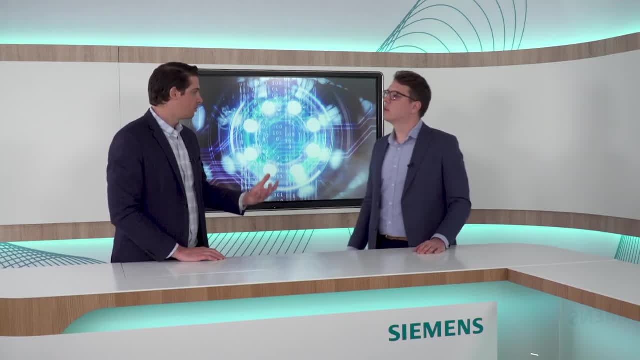 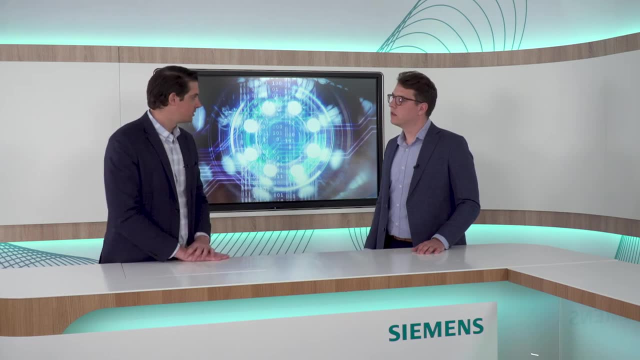 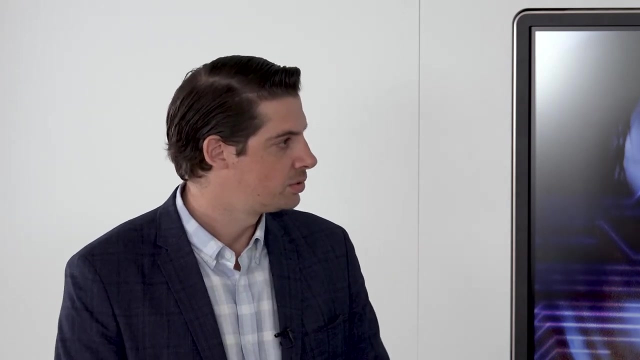 So ASHRAE, as one of the most prevalent industry groups, representing the building control industry in particular, are starting to join with these smart guys that you talked about to really start to build this into the core of our individual and independent industry approach. 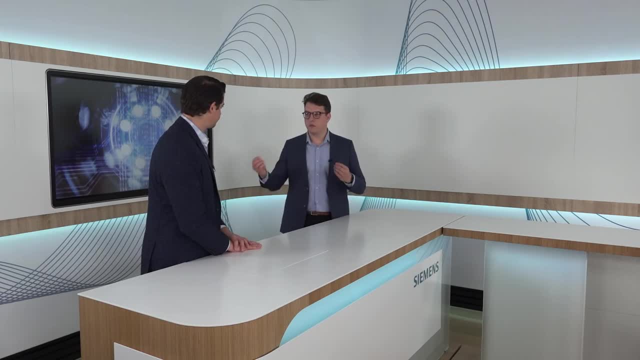 Exactly. And they're just saying like, okay, we've got all this great data, We've got all these great systems popping out. Now we're combining the industry knowledge with people straight out of university and saying these data scientists or computer scientists or 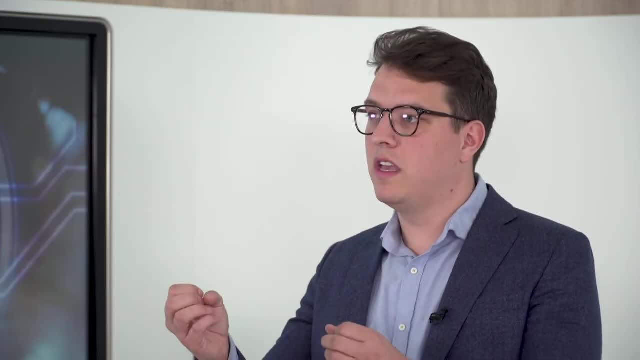 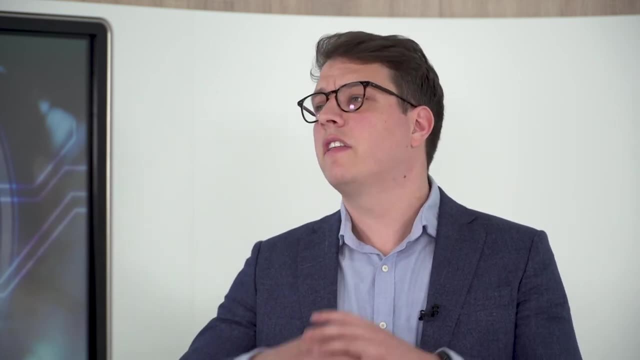 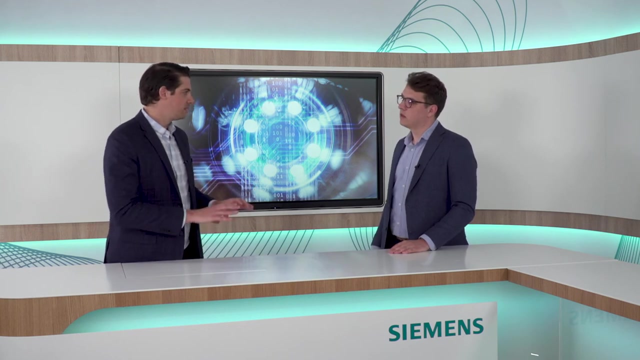 mathematicians. how can we solve this problem? How can we have something that our industry can grab and utilize And that will then go into all the hardware we sell, into anything that we install into any building? So semantic tagging and semantic data models are ways for us to embed information within data that 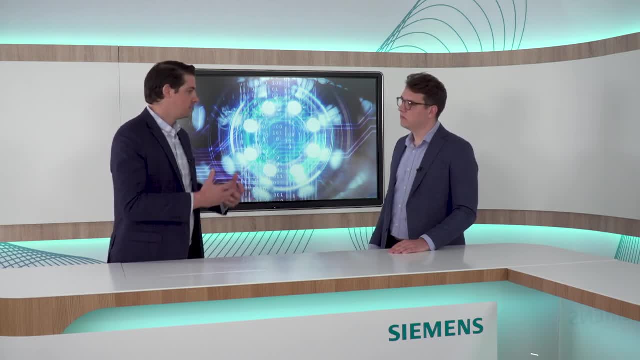 identifies what it is and what its purpose is, so that we can more easily sift through the huge pile, this huge lake of information that we're collecting, and find the things that we need to make, the decisions that we'd like to derive Exactly, And all the relationships tied to that piece. 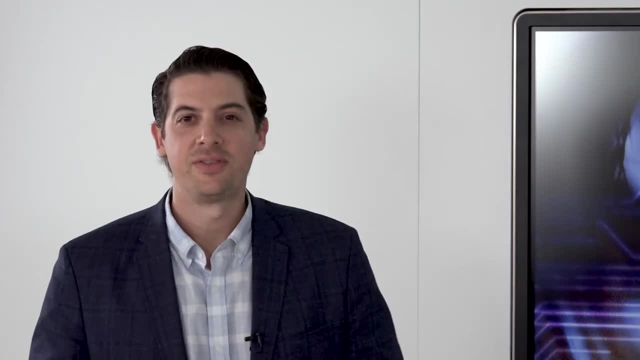 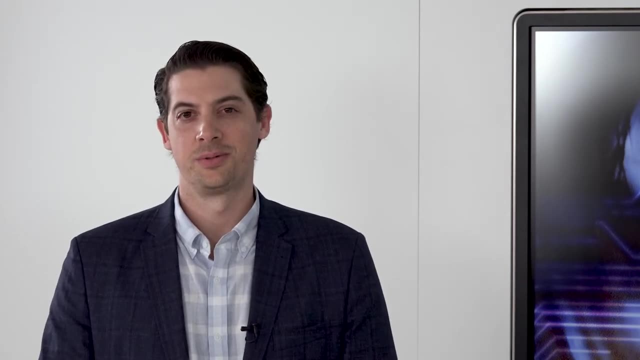 And all the relationships tied to that piece of data as well. Perfect, Thank you very much. Thank you, And thank you all for joining us here on Buildings of Tomorrow. Please feel free to like, comment or share this episode, and also ensure to subscribe to us here on.